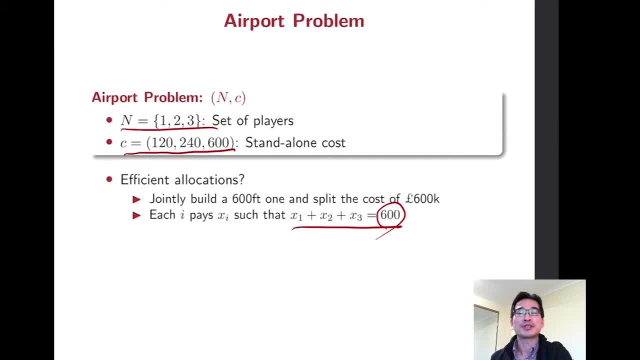 So the sum of payment is 600, then that's efficient allocation. So we can consider very naive cost allocation. For instance, they can split the cost equally, But this is not good because airline 1 will block this allocation, because airline 1 can build its own runway and it just costs 120. So this airline 1 has no incentive. 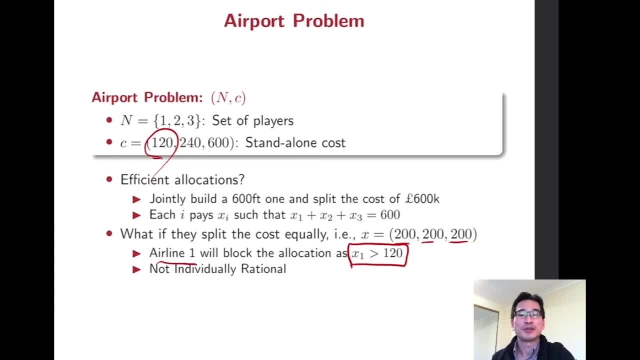 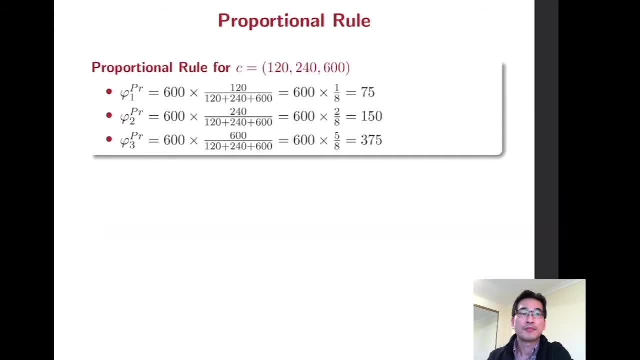 to participate in this coalition, Then this is not individually rational. So this allocation is not fair. Any of you may think proportional rule might be good. So the sum of this standard of cost is 960.. So the smallest airline company pays 120 divided by. 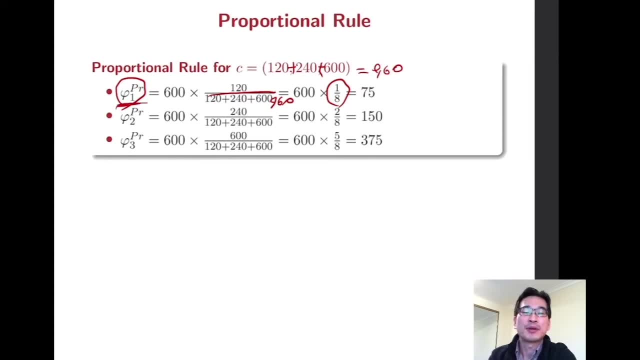 960, which is 1: eighth. So this company- The proportion of thistı- pays 1: 8th of 600, and the second company pays 2: 8th, which is proportional to the sum of individual cost, and the largest one pays 5: 8th. so this is the payment. 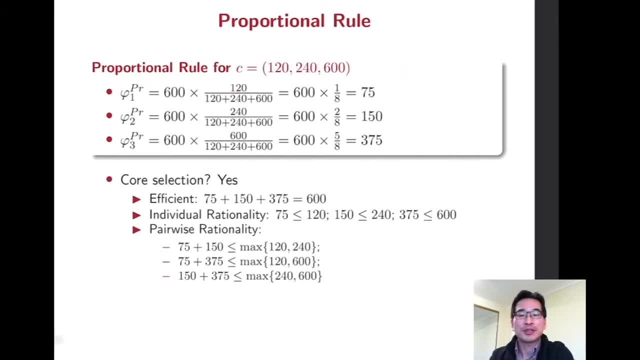 based on proportional rule. so you can check this allocation. this payment rule satisfies core location, so this is core selection. so efficiency. you can see the sum of their payment is 600, so it's efficient and individual rationale. so the first company pays 75, which is less than standalone cost, and the second 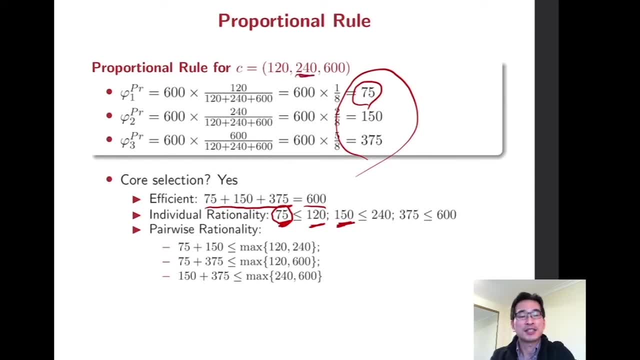 one pays 150 less than is standalone cost and the larger one pays 375, which is lower than is standard or cost at 600. so it's individually rational and you can also find that is pairwise rational. so sum of the first two companies payment 75 plus. 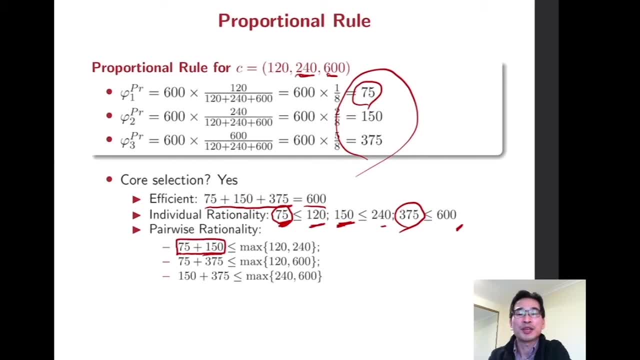 percent. 150 is smaller than the cost of the largest runway, 240, and the sum of the payment of first and third, that is, is smaller than 600, which is less than standalone cost. and that's pairwise here and this time you what the first and third requires jointly and second and third also their 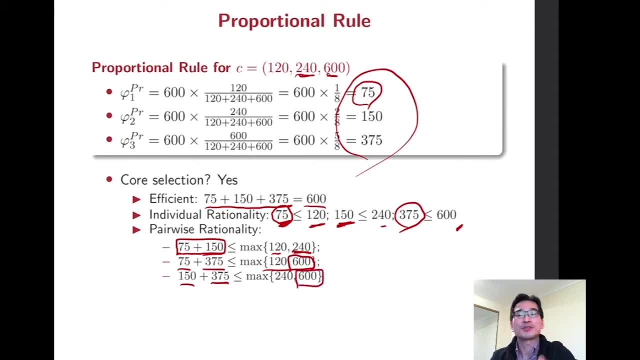 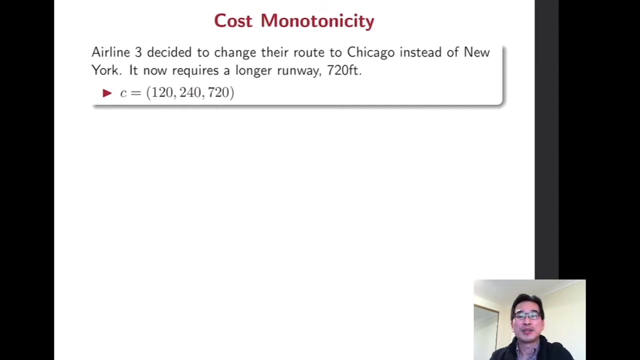 payment. some of the payment is smaller than 600, so that satisfies pairwise resort. so we can confirm this proportional rule is in quo. so can we say: is it fair? but there are many other properties or action for fairness. now let's think about another situation. so airline 3 decide to change their route. 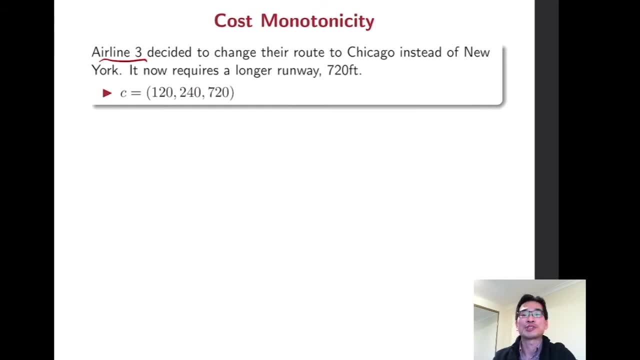 to Chicago instead of New York. so it requires a longer runway, say it requires 720 feet. so now the cost function. so standalone cost is 120 and 240 and 720. so first the company didn't change it their cost, but the last company requires more cost. 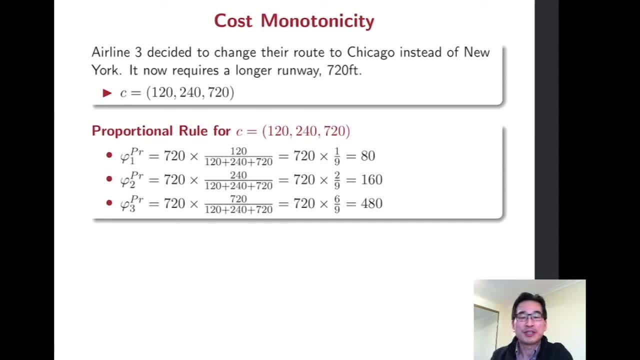 So again, let's apply the proportional rule. So everything's are the same, but this denominator is different, And the first one is supposed to pay one ninth of the total cost, And the second one pays two ninths, and third one pays six ninths of the total cost: 720.. 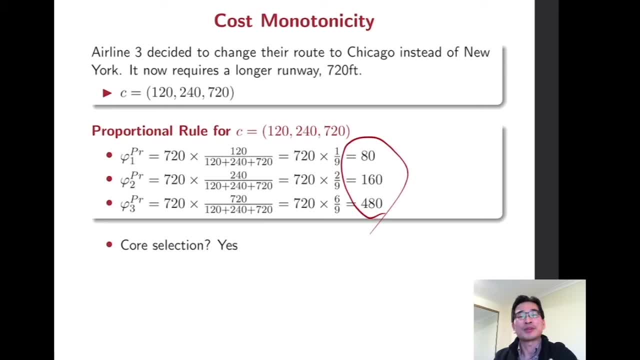 So still, you can see this payment is in the core by looking at the individual rationality and efficiency and the parallelized rationality. But compared to the original situation- airline one and airline two- they are required to pay more, Although they do not use that additional part of the runway. 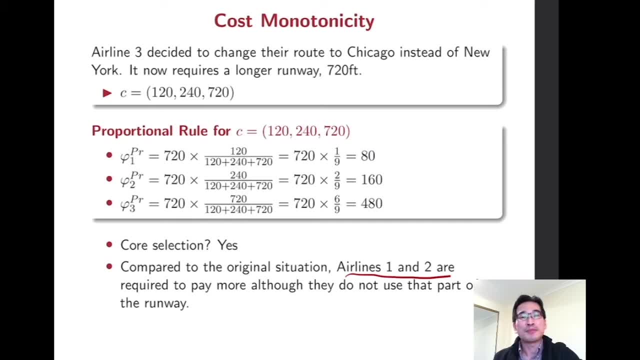 So the airline one and airline two may consider this situation is not fair. So a good solution may have a desired property across different situations. So in that sense proportional rule is not fair. So now we are going to consider. So now we are going to consider. 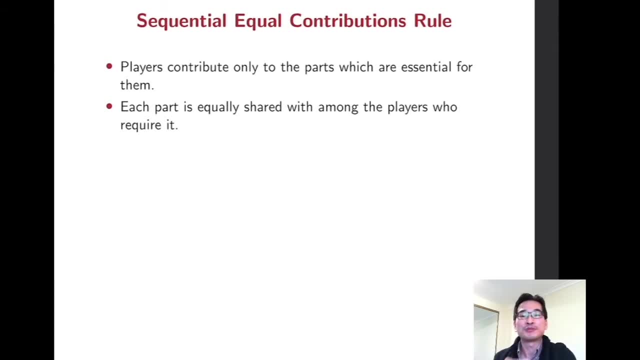 Another allocation rule that is sequential equal contributions rule. So players contribute only to the parts which are essential for them And each part is equally shared among the players who require it. So we need to construct 600.. So we need to construct 600.. 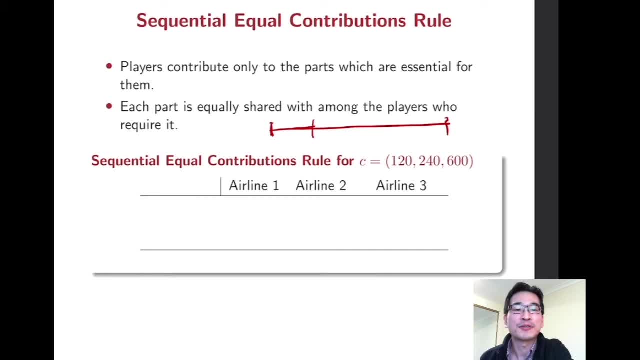 And first 120.. And this part is required by all 3 airlines. And this part is required by all 3 airlines. So this first part split equally. The cost is going to be split equally And the second rule is that 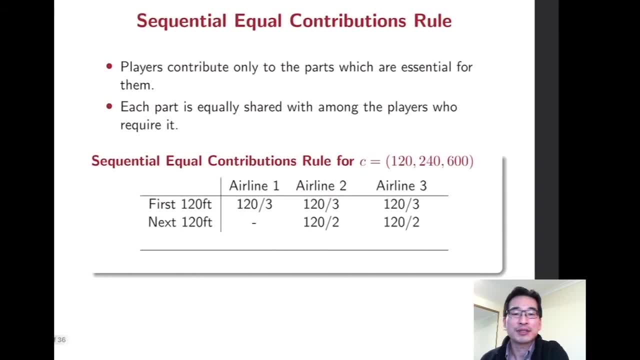 The cost is going to be split equally. The second part, so the first airline company, second and third, they all use this part And the second part the first airline company is not going to use The additional 120 is only used by second and third one. 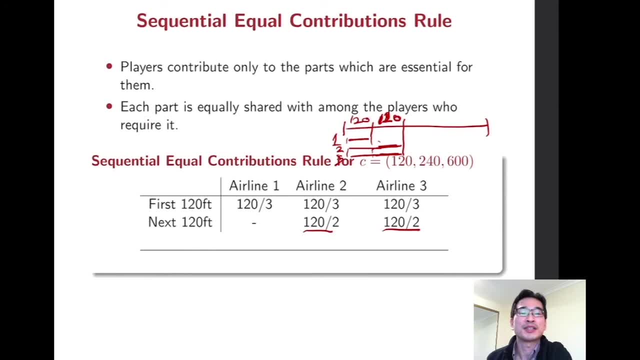 So the second and third one split the additional cost equally, And now the remaining part is 360, and only the third airline company will require this part. For this part, only airline company three will pay. So this is the allocation based on sequential equal contributions rule. 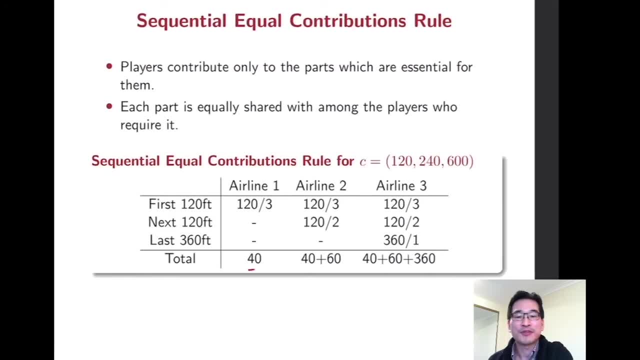 So what's the total? So the first airline company, First airline company- pays 40, and second one pays 40 for the first part and 60 for the second part. And the largest airline company pays 40 for the first part and 60 for the second part. 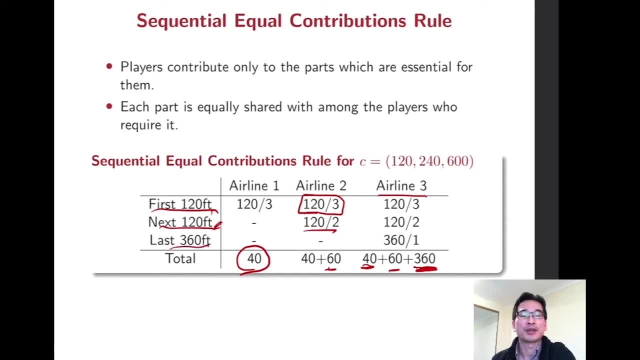 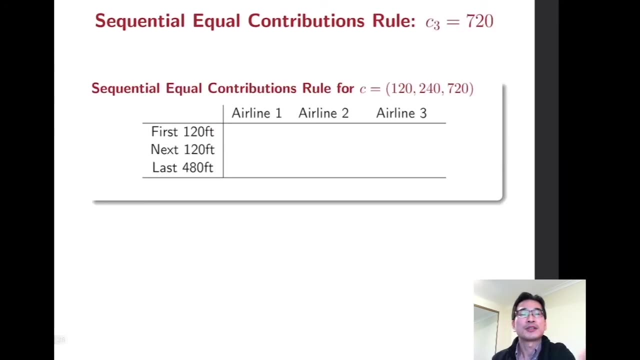 and 360 for the last part. So their payment is 40,, 100, and 460. And you can easily Check. This is in the core And again, we can do the same exercise with different cost, in which the largest airline 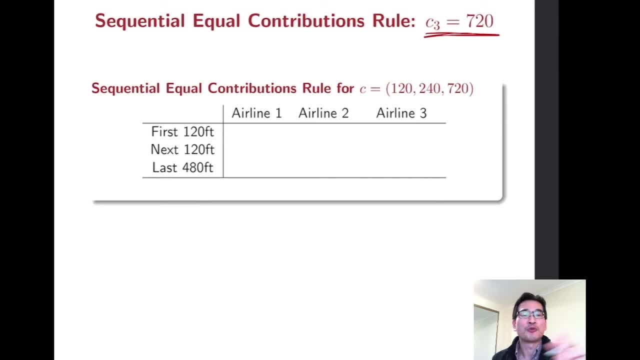 requires a little bit more runway. So first part again split equally among the three players. And second part: split equally among the three players And the third one And second part. 120, split equally between airline two and airline three. 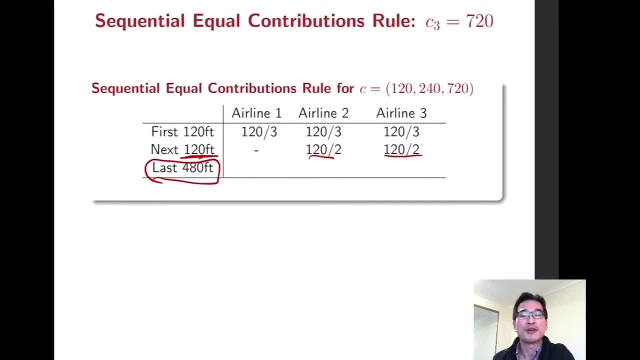 And last part. the remaining part is 480.. So the increased part, the additional part, is only responsible for last airline company. So the first and second company. So the first and second company. So the last airline company. So the first and second company. 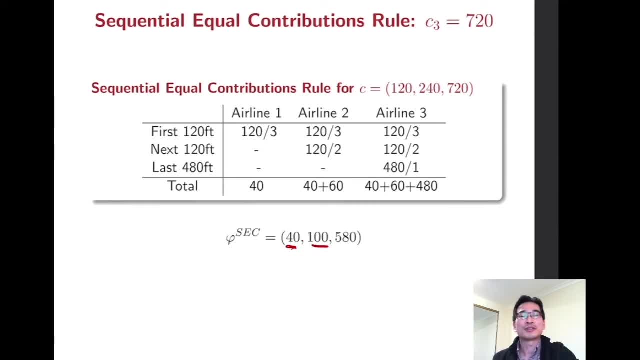 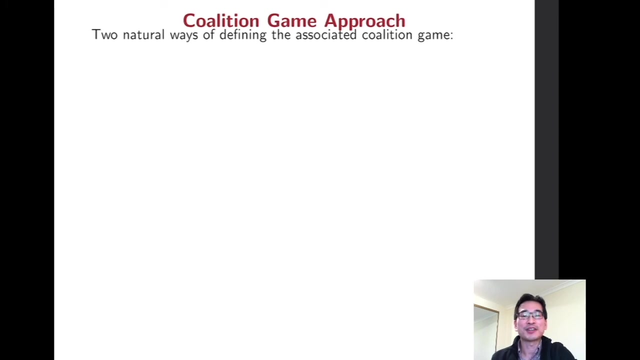 company. their payment did not change and only the last player should pay more. So in that sense, sequential equal contribution rule is better or fairer than proportional rule. Now let's define coalition game based on this situation. So there are two natural ways of defining the associated coalition game. 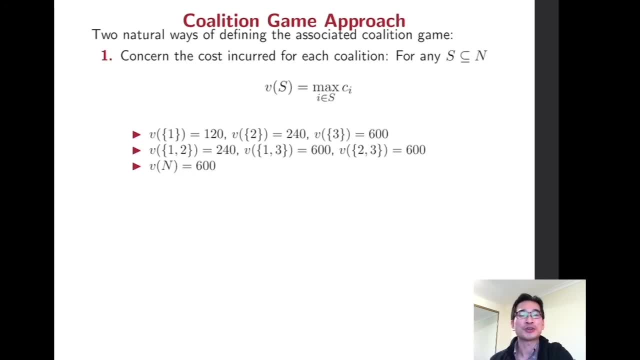 The first one is to concern the cost incurred for each coalition, So this characteristic function is the maximum cost of each individual's stand-alone cost. So V of 1 is 120,, V of 2 is 240, and V of 3 is 600. So V of 1 is 120, V of 2 is 240, and V of 3 is 600.. So V of 1 is 120, V of 2 is 240, and V of 3 is 600.. 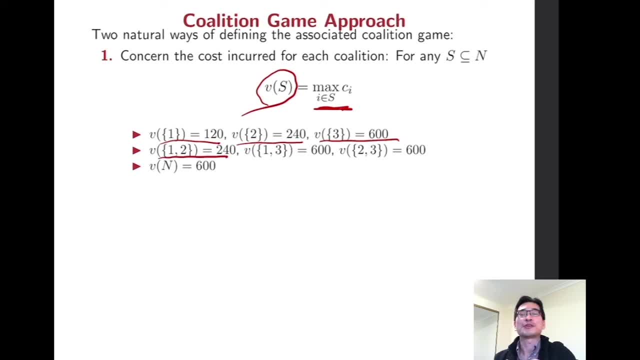 By forming 1 and 2, they'll have to pay 240.. By forming 1, 3, they have to pay 600.. By forming 1, 3, they have to pay 600.. By forming 1,, 2, 3, it still requires 600. 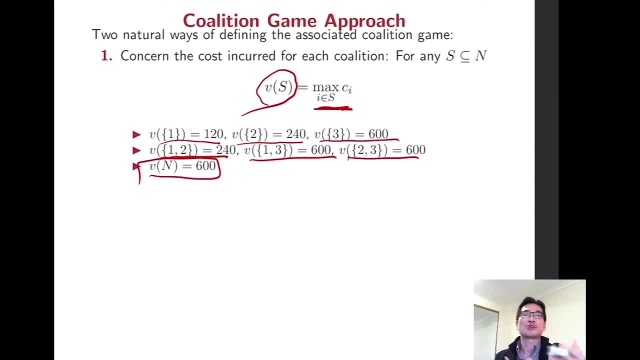 By forming 1,, 2, 3,, it requires 600.. By forming 1,, 2, 3,, it still requires 600.. So this is one way of defining coalition game, if it makes sense, And another way to define a coalition game is to judge its tied, defensiveness and outside. 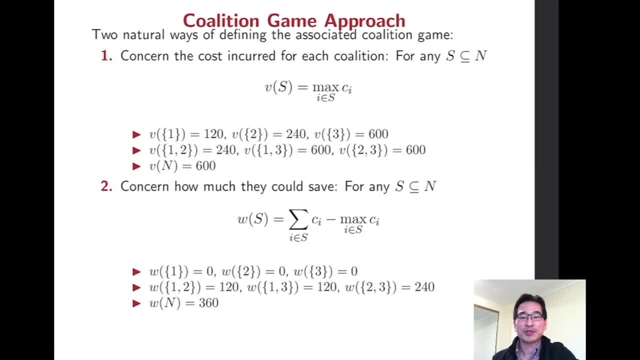 approach is considering how much they could save by forming a coalition. So now we define different characteristic function: the difference between the sum of individual cost- what they have to pay if they build the runways separately- and the maximum of the cost. 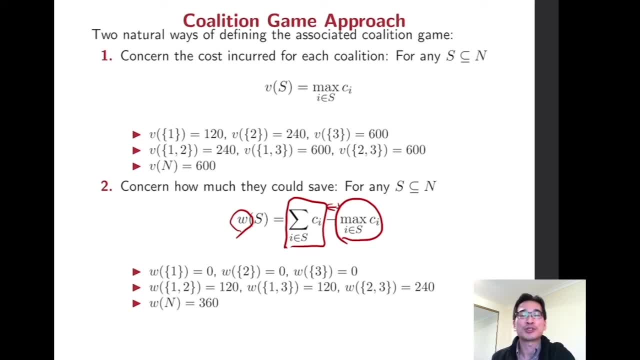 So this difference is the how much they could save. So, each individual, they can save nothing, and by forming a coalition they can save $120 and $180.. forming a coalition 1-3, they can save 120.. By forming a coalition 2-3, they can. 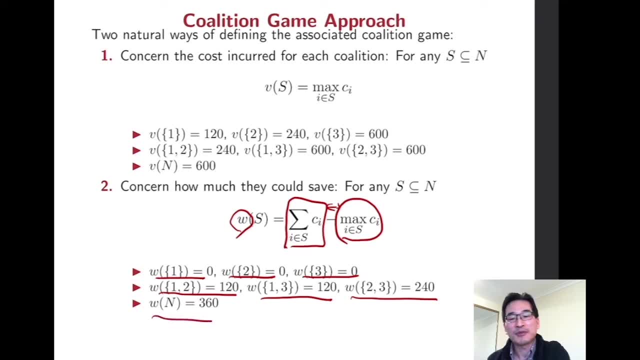 save 240.. And by forming a grand coalition they can save 360.. This is another way of defining the coalition game. It might be good if a solution is the same allocation to different versions of a coalition game, If a solution is robust to the way of defining a coalition game. 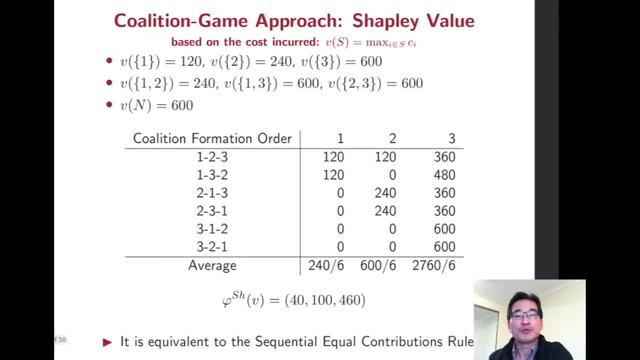 then the solution might be good. Now we are going to find the share-free value to this coalition game, Based on the cost incurred. the first approach- And I'm going to skip the detail, but you can check the share-free value of this coalition game we defined. 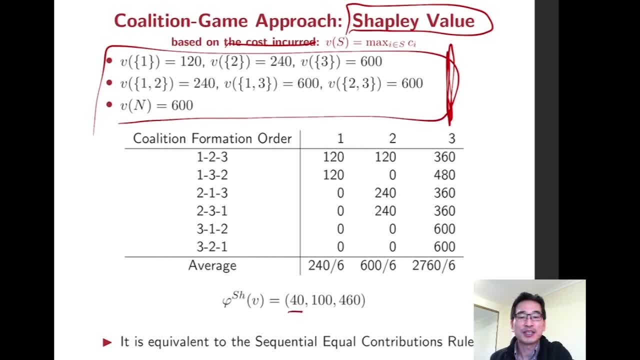 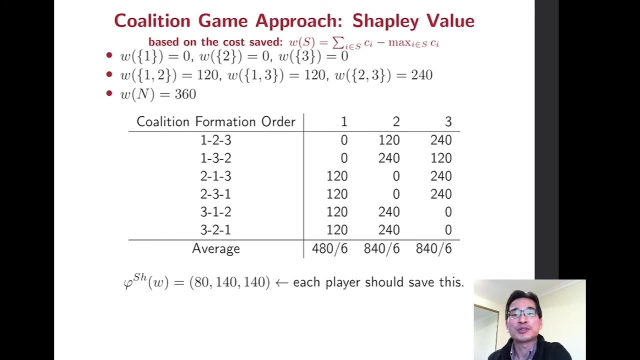 is 40,, 100, and 460.. That is equivalent to the sequential equal contributions rule. Also, if we consider another approach, we can say: this is 40, 100, and 460.. This number of names of players we can use to determine the share-free value.